if we multiply that by x1 and x2, we get a 0 in for xp. If we multiply that by x1 and x2, we get a 0 in for xp. If we multiply that by x1 and x2, we get a 0 in for xp If we multiply that by x1 and x2,. 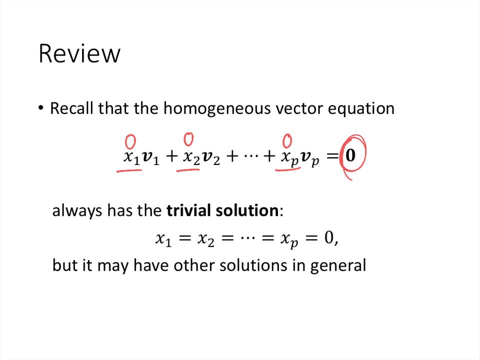 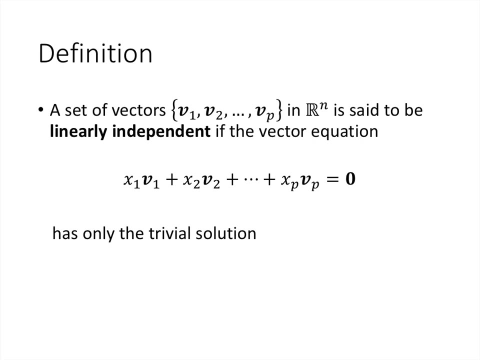 all of those v vectors by 0 and add up the results, of course we will get the 0 vector. But as we've talked about, this homogeneous equation may have more solutions. So now let's get to the definition. So if we have a set of vectors, v1 through vp, all living in Rn, 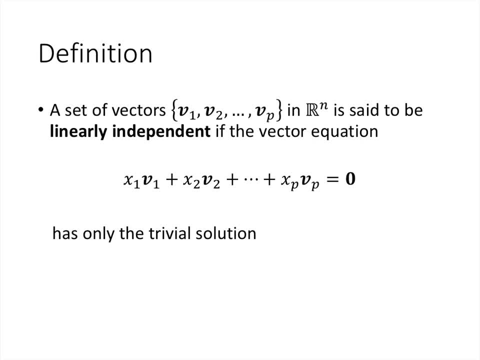 so that just means that those vectors have n entries. we say that this set of vectors is linearly independent if that homogeneous vector equation only has the trivial solution. So if setting all of the x's equal to 0 is the only way to make the left-hand side equal the right-hand. 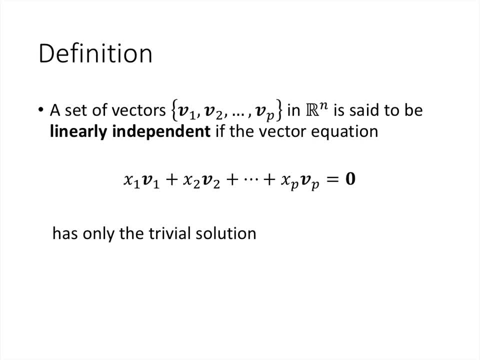 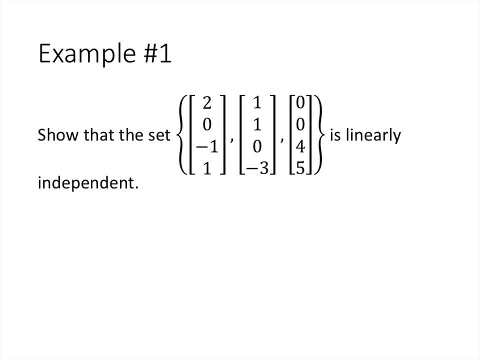 side. then we say that the vectors that we started with were linearly independent. So here's an example. We've got three vectors here. We want to show that the set of vectors is linearly independent. So we're going to call our first vector v1,, our second vector, v2,. 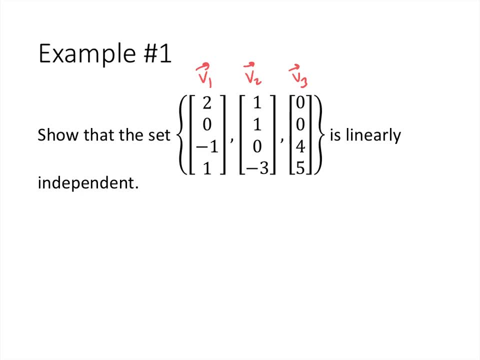 and our third vector, v3.. So the vector equation that we're talking about looks like x1, v1 plus x2, v2 plus x3, v3 equals the 0 vector. So in other words, x1 times the vector 2: 0 negative. 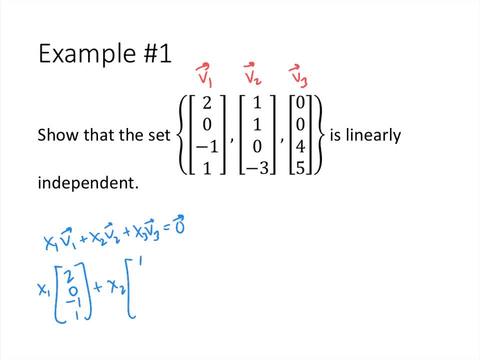 1, 1 plus x2 times the vector 1, 1, 0 negative 3 plus x3 times the vector 0, 0, 4, 5, and that's being set equal to the 0 vector. Now we've talked about how we can solve this vector equation. 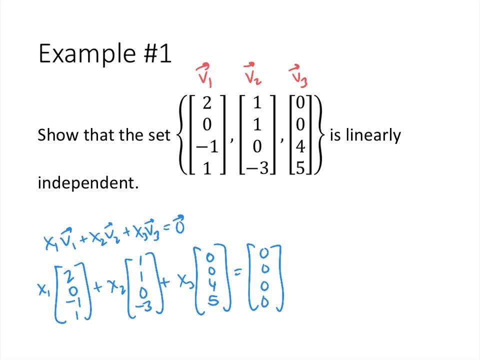 very similarly to how we solve a system of linear equations, and that's by setting up an augmented matrix. So the augmented matrix that we would get looks like 2: 0 negative 1, 1,. 1, 1, 0 negative 3,. 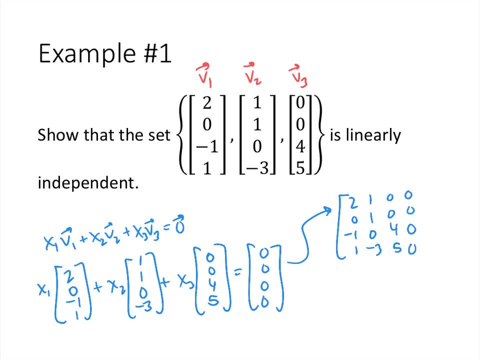 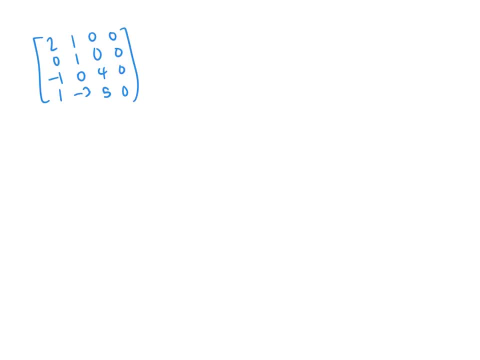 0, 0, 4, 5, and then a column of zeros. So that's our augmented matrix, and now let's work to row reduce that. Sometimes we skip over the row reduction, but let's actually work it out this time. So we'll start by multiplying the first row by one half. 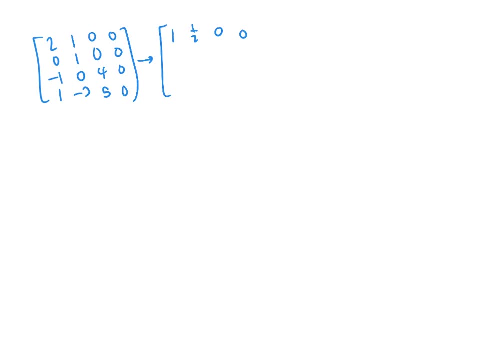 That gives us 1, 1 half 0, 0 across the top The first column. a second entry already has a 0, so we'll leave that alone. And now let's multiply the first row by 1 and add it to the third row. 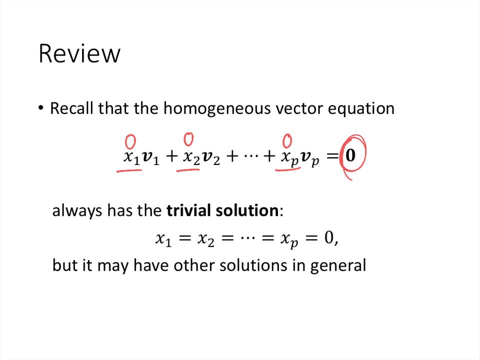 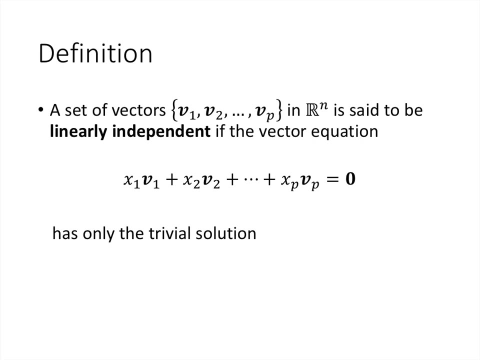 if we multiply all of those v vectors by 0 and add up the results, of course we will get the 0 vector. But as we've talked about, this homogeneous equation may have more solutions. So now let's get to the definition. So if we have a set of vectors, v1 through vp, all living in Rn, 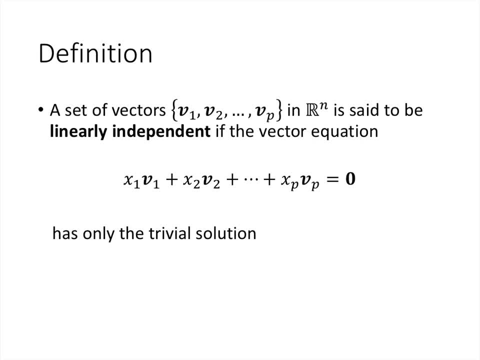 so that just means that those vectors have n entries. we say that this set of vectors is linearly independent if that homogeneous vector equation only has the trivial solution. So if setting all of the x's equal to 0 is the only way to make the left-hand side equal the right-hand. 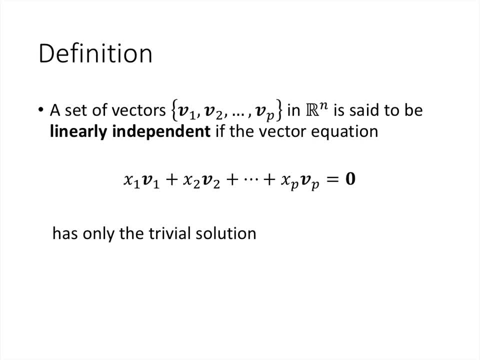 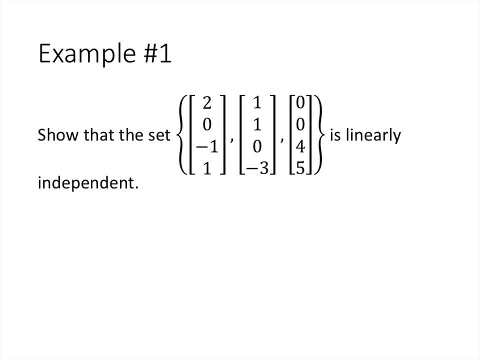 side. then we say that the vectors that we started with were linearly independent. So here's an example. We've got three vectors here. We want to show that this set of vectors is linearly independent. So we're going to call our first vector v1,, our second vector, v2,. 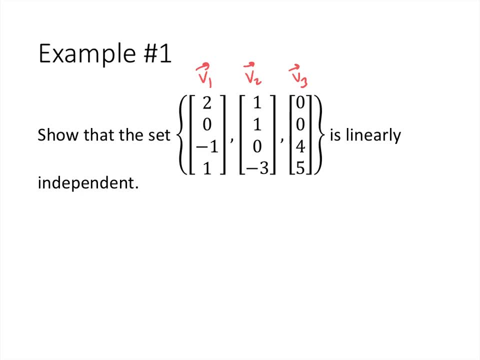 and our third vector, v3.. So the vector equation that we're talking about looks like x1, v1 plus x2, v2 plus x3, v3 equals the 0 vector. So in other words, x1 times the vector 2: 0 negative. 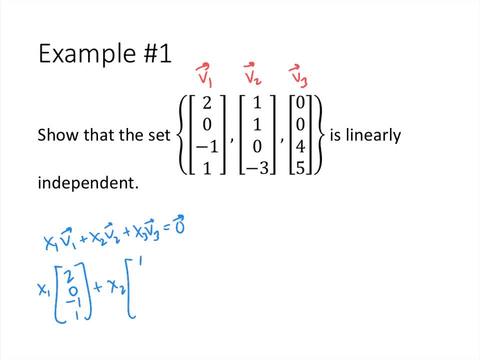 1, 1 plus x2 times the vector 1, 1, 0 negative 3 plus x3 times the vector 0, 0, 4, 5, and that's being set equal to the 0 vector. Now we've talked about how we can solve this vector equation. 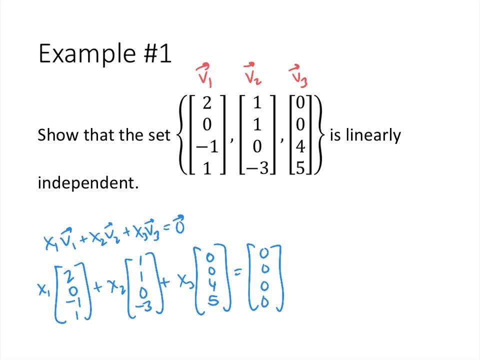 very similarly to how we solve a system of linear equations, and that's by setting up an augmented matrix. So the augmented matrix that we would get looks like 2: 0 negative 1, 1,. 1, 1, 0 negative 3,. 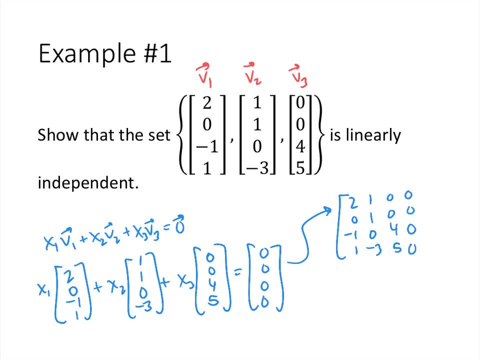 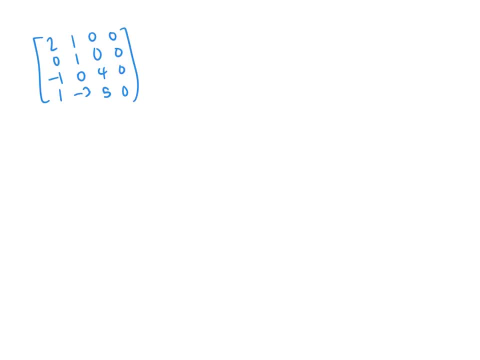 0, 0, 4, 5, and then a column of zeros. So that's our augmented matrix, and now let's work to row reduce that. Sometimes we skip over the row reduction, but let's actually work it out this time. So we'll start by multiplying the first row by one half. 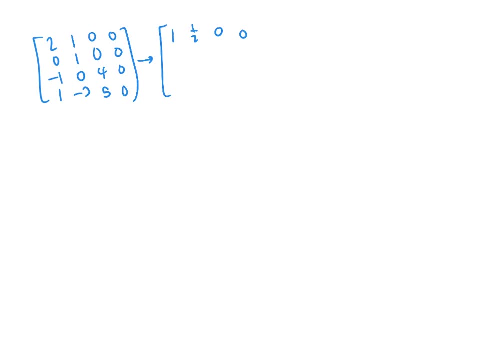 That gives us 1, 1 half 0, 0 across the top The first column. a second entry already has a 0, so we'll leave that alone. And now let's multiply the first row by 1 and add it to the third row. 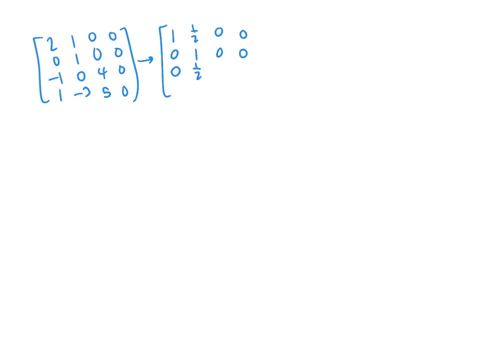 That gives us 0,, 1, half 4,, 0.. And then let's multiply the first row by negative 1 and add it to the fourth row, That gives us 0.. Negative half plus 3 is negative 7 over 2, and then 5, and then 0.. 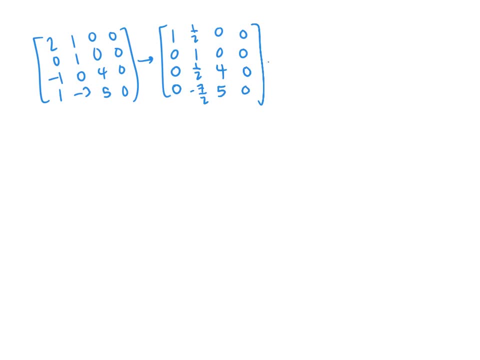 Continuing. we already have a 1 in the second row, second column, so we'll leave that alone. Our first column is going to be locked in and we're not changing the second row in this step. So we'll multiply the second row by negative a half and add it to the first row. That's just. 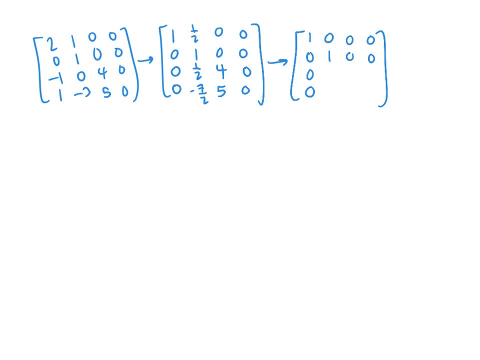 going to give us a 0 there and a 0 and a 0. Again, multiply by negative a half and add it to the third row. That's going to give us a 0 here. Still, we have a 4 and a 0. And then we'll multiply. 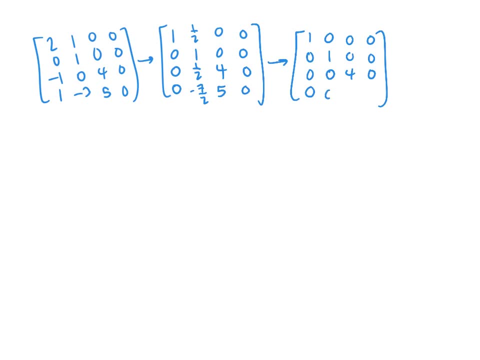 the second row by 7 halves and add it to the fourth row. That'll just cancel out the second row, Cancel out the 7 halves and we'll still have a 5 and a 0.. A couple more steps. Multiply the third. 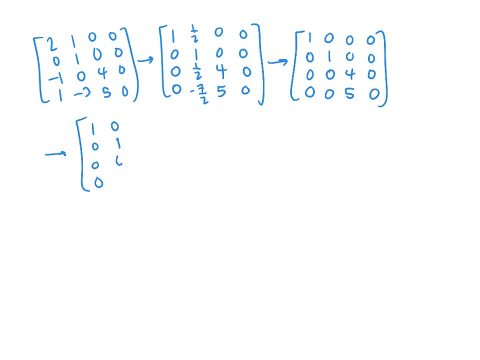 row by 1. fourth, That's going to give us a 1.. The rest of the third column looks good, and then we'll multiply the third row by negative 5 and add it to the last row. That's just going to cancel out that. 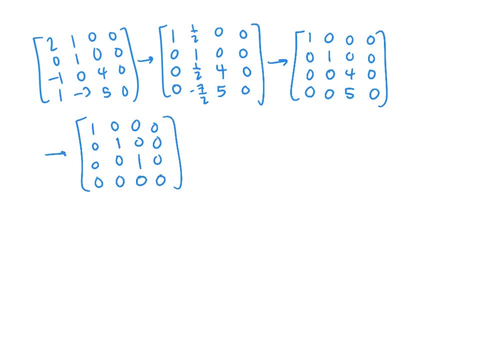 5, and so here's our row-reduced matrix. Now we translate this back into the language of equations. So remember, we've got our equation and we're going to have a 1., And then we're going to have a 2., And then we're going to have a. 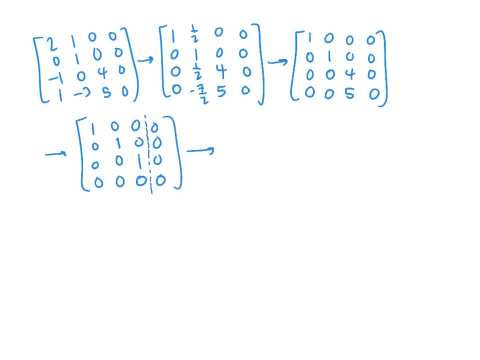 matrix here, so that last column represents the right-hand side of the equal sign. So this is just telling us: x1 equals 0, x2 equals 0, x3 equals 0.. We didn't have any free variables, so we don't have any additional solutions. All we have is this trivial solution. So the trivial 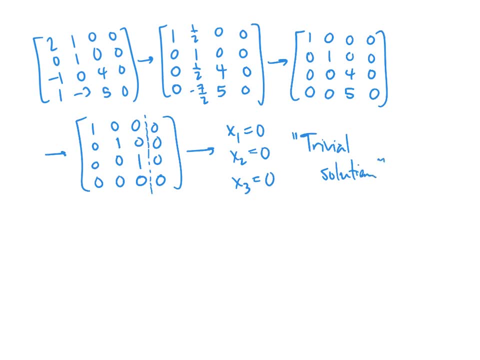 solution is just our name for the solution that we know we always have. we just sometimes have more than just this solution. But in this case, for these equations, all we had was the trivial solution, and that's what we need to show if we want to show that those vectors are linearly. 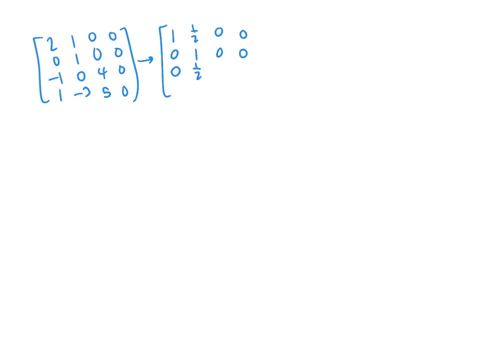 That gives us 0,, 1, half 4,, 0.. And then let's multiply the first row by negative 1 and add it to the fourth row, That gives us 0.. Negative half plus 3 is negative 7 over 2, and then 5, and then 0.. 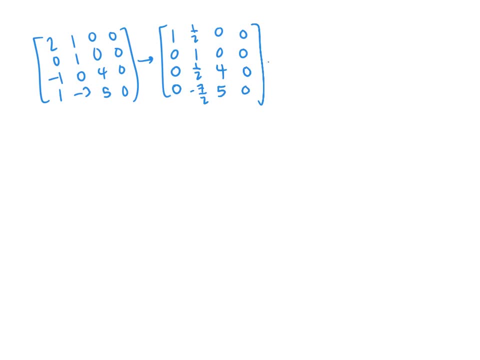 Continuing. we already have a 1 in the second row, second column, so we'll leave that alone. Our first column is going to be locked in and we're not changing the second row in this step. So we'll multiply the second row by negative a half and add it to the first row. That's just. 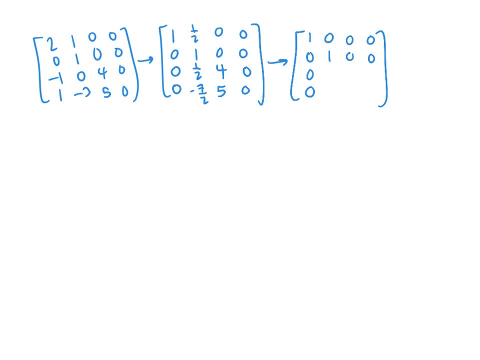 going to give us a 0 there and a 0 and a 0. Again, multiply by negative a half and add it to the third row. That's going to give us a 0 here. Still, we have a 4 and a 0. And then we'll multiply. 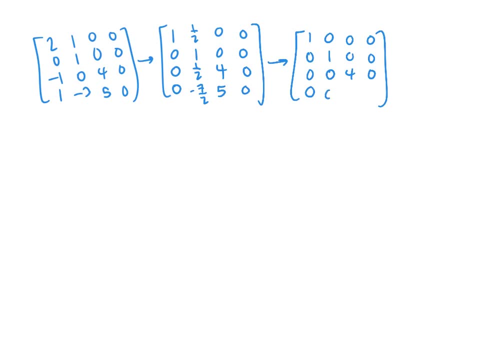 the second row by 7 halves and add it to the fourth row. That'll just cancel out the first row. We'll still have the 5 and a 0.. A couple more steps: Multiply the third row by 1 fourth. That's going to give us a 1.. The rest of the third column looks good, and then we'll multiply the. 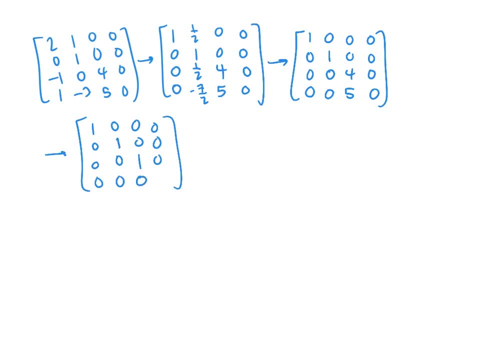 third row by negative 5 and add it to the last row. That's just going to cancel out that 5, and so here's our row-reduce matrix. Now we translate this back into the language of equations. so remember, we've got our. 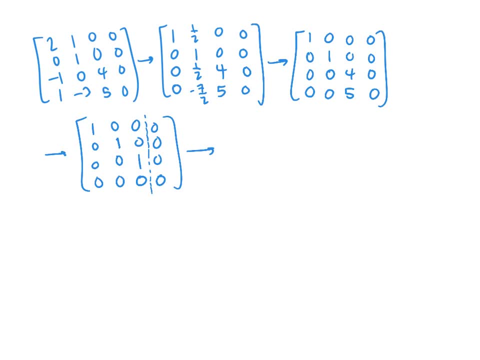 augmented matrix here, so that last column represents the right-hand side of the equal sign. So this is just telling us: x1 equals 0, x2 equals 0, x3 equals 0.. We didn't have any free variables, so we don't have any additional solutions. All we have is this trivial solution. So the trivial. 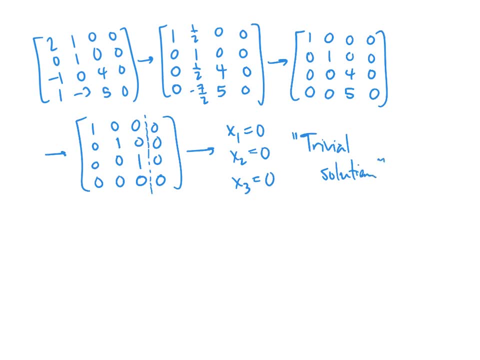 solution is just our name for the solution that we know we always have. we just sometimes have more than just this solution. But in this case, for these equations, all we had was the trivial solution, and that's what we need to show if we want to show that those vectors are linearly. 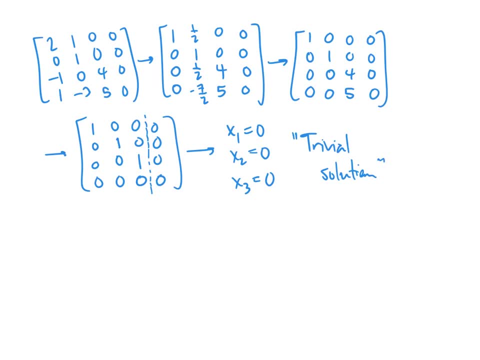 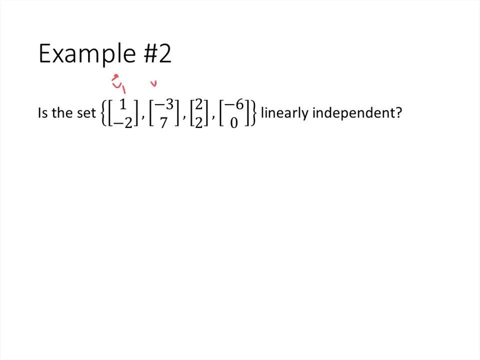 independent. Let's do another example. This time we have four vectors, so we'll call them v1, v2, v3, and v4.. The vector equation we're talking about is x1, v1 plus x2, v2 plus x3, v3 plus x4, v4,. 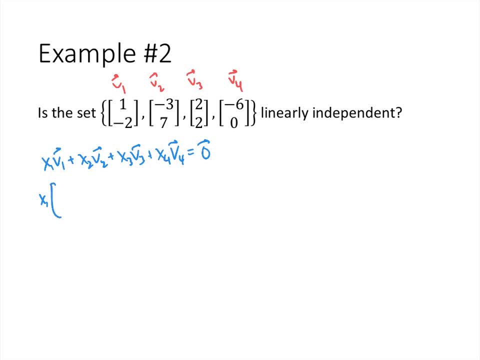 equals the 0 vector Plugging in our vectors we have 1, negative, 2, negative 3, 7, 2, 2, and negative 6, 0. Now we set up the corresponding augmented matrix which looks like 1, negative, 2,. 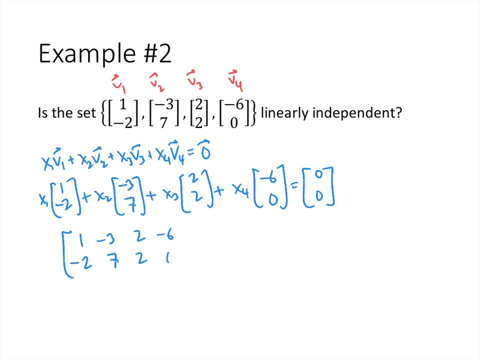 negative 3, 7, 2, 2, negative 6, 0, 0, 0.. We've got a 1 in the first row, first column, so we'll just take that first row and multiply it by 2 and add it to the second row, So we get 1, 0.. We're not. 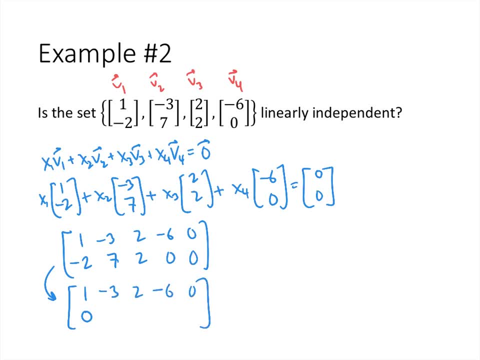 changing the first row. Negative 3 times 2 plus 7 is 1.. 2 times 2 is 4 plus 2 is 6.. Negative 6 times 2 is negative 12, and we get a 0.. For this to be in reduced 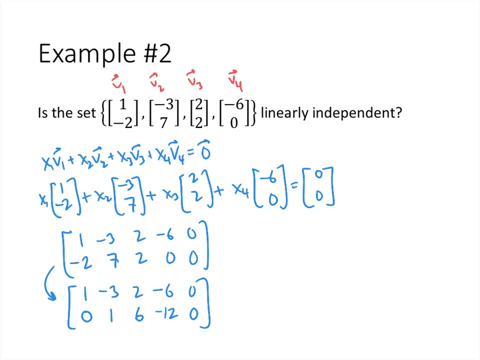 echelon form. we know that we need to multiply the second row by 3 and add it to the first row. 6 times 3 is 18 plus 2 is 20.. Negative 12 times 3 is negative 36, plus negative 6 is negative 42, and we get a 0.. And now every row has a pivot. 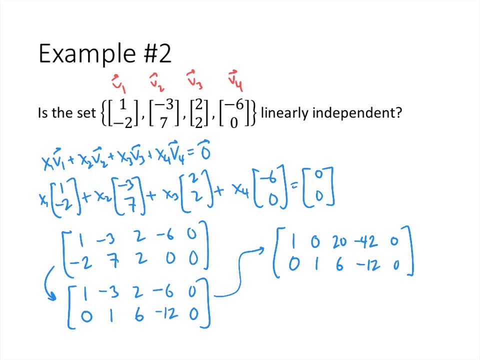 There's nothing else we can do to reduce this matrix any further. This is in row reduced echelon form. But now notice that x3 and x4 are free variables And that means that this vector equation has non-trivial solutions. It's got a different solution for each value of x3 and x4 that we 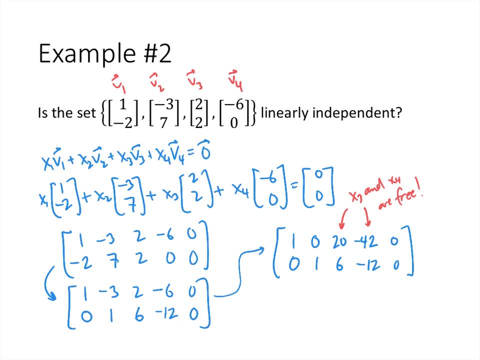 might choose. So this vector equation has lots of solutions, and so certainly it has more than just the trivial solution. So the answer to the question: are these vectors linearly independent? is no. Linearly independent means the only solution we found was the trivial solution. 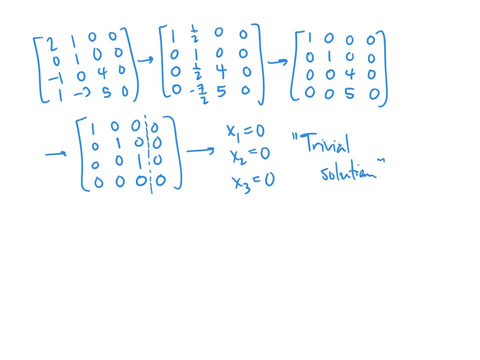 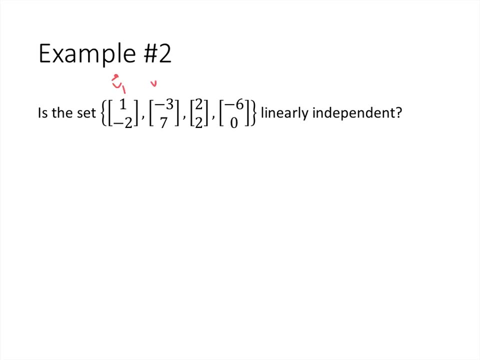 independent. Let's do another example. This time we have four vectors, so we'll call them v1, v2, v3, and v4.. The vector equation we're talking about is x1, v1 plus x2, v2 plus x3, v3 plus x4, v4. 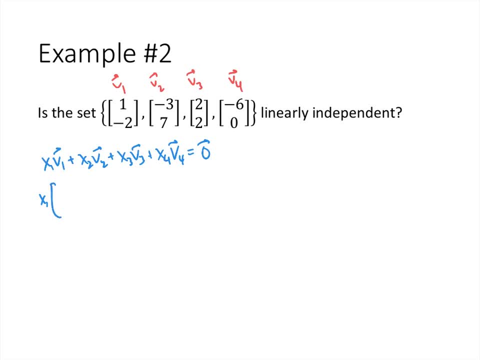 equals the zero vector Plugging in our vectors we have 1, negative, 2, negative 3, 7, 2, 2, and negative 6, 0. Now we set up the corresponding augmented matrix which looks like 1, negative, 2,. 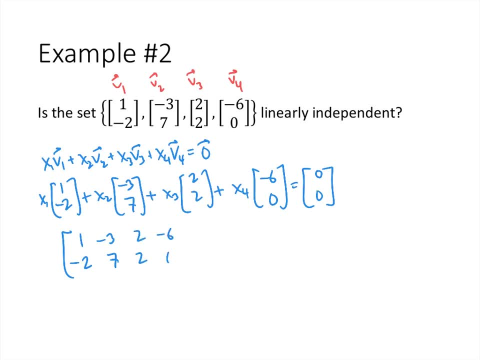 negative 3, 7, 2, 2, negative 6, 0, 0.. We've got a 1 in the first row, first column, so we'll just take that first row and multiply it by 2 and add it to the second row, So we get 1, 0.. We're not changing the first row. Negative 3 times. 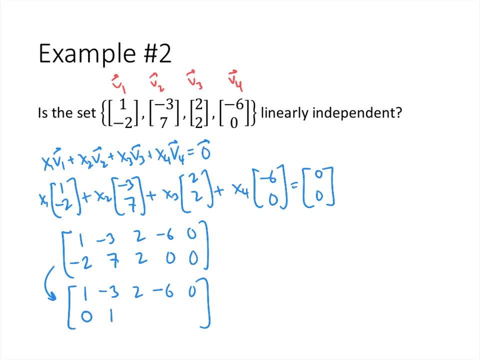 2 plus 7 is 1.. 2 times 2 is 4, plus 2 is 6.. Negative 6 times 2 is negative 12, and we get a 0.. For this to be in reduced echelon form, we know that we need to multiply the second row by 3 and add it to the. 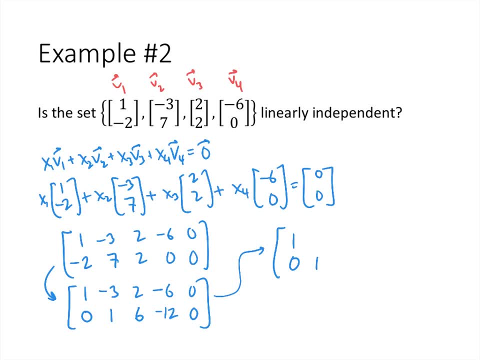 first row: 6 times 3 is 18 plus 2 is 20.. Negative 12 times 3 is negative 36. plus negative 6 is negative 42, and we get a 0.. And now every row has a pivot. There's nothing else we can do to. 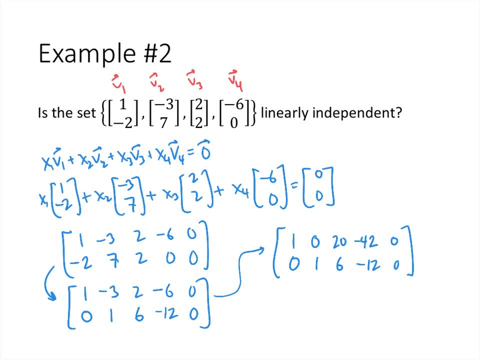 reduce this matrix any further. This is in row-reduced echelon form. But now notice that x3 and x4 are free variables And that means that this vector equation has non-trivial solutions. It's got a different solution for each value of x3 and x4 that we might choose. So this vector equation 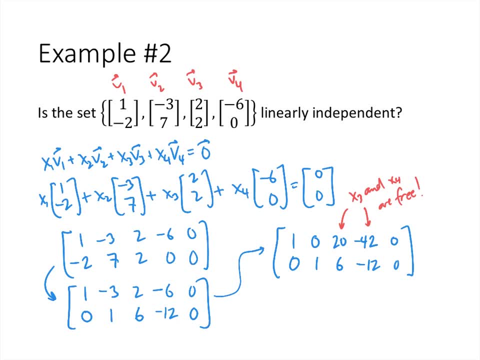 has lots of solutions and so certainly it has more than just the trivial solution. So the answer to the question: are these vectors linearly independent? is no, Linearly independent means the only solution we found was the trivial solution. In this case we found lots of solutions, so that means that the vectors are not linearly. 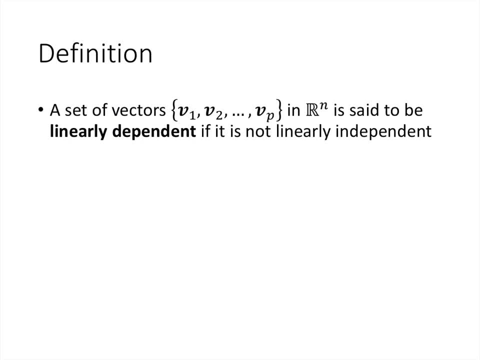 independent. So this gives us another piece of terminology. We can flip around the definition of linear independence and talk about what it means for a set of vectors to be linearly dependent. So linearly dependent just means not independent, It's the opposite of the word. 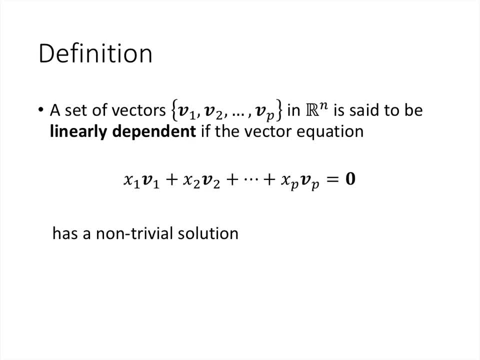 independent. We can be more specific though, Putting in the definition of linear independence. if we say that the linearly dependent means that the vectors are not linearly independent, then that just means that that vector equation has a non-trivial solution. Remember linear. 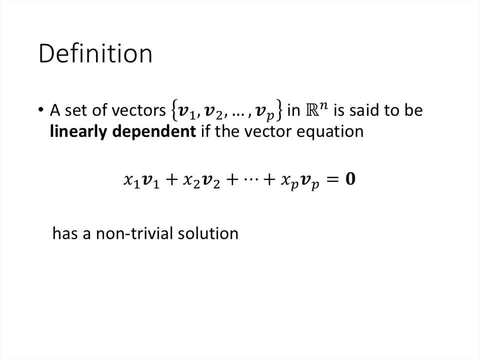 independence means that the only solution is the trivial solution. So linearly dependent would mean that there is at least one other solution other than the trivial solution. Being a little bit more specific, what linearly dependent means is that there are some numbers that exist that exist, that are not all zero. some of them might be zero. 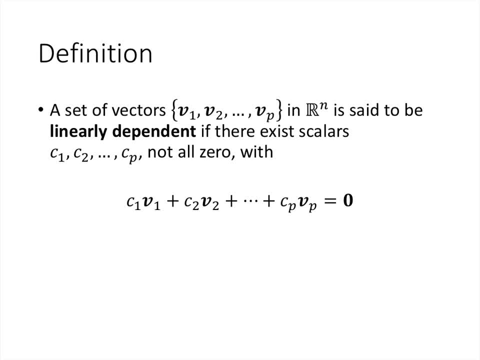 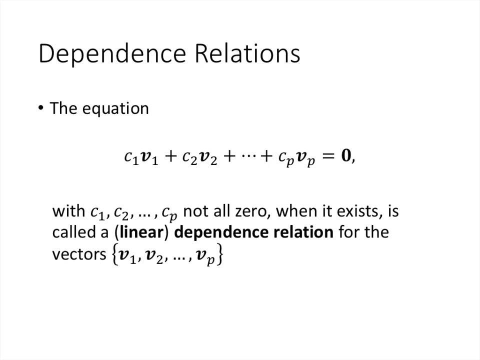 but they're not all zero- that we could plug in for the x's to make that linear combination end up being the zero vector. And this equation here has a special name. We call that equation a dependence relation or a linear dependence relation for those vectors. 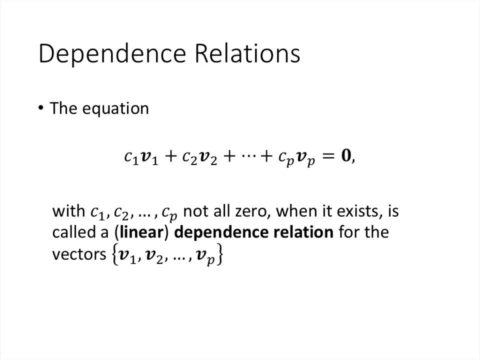 If there's some way to plug in numbers for the x's that are not all zero, tend to be this one: make the left hand side equal the right hand side. That way of doing that is called a dependence relation and in general, for a set of vectors that are: 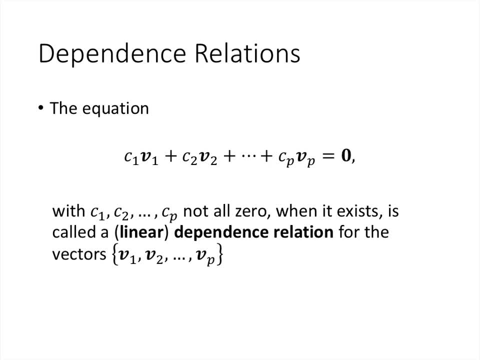 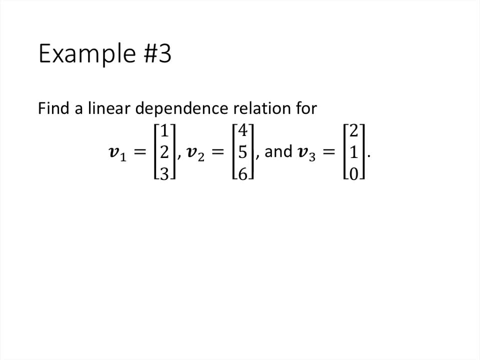 linearly dependent. there are lots of ways to do that. Let's do an example. So here we have three vectors. Now I'm telling you that these vectors are linearly dependent, although we'll see that for ourselves as we go through this example. but given these three vectors, what we want to find is a linear 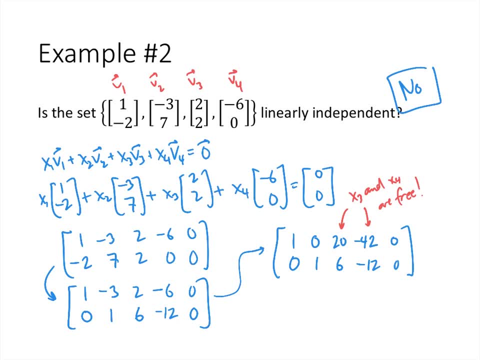 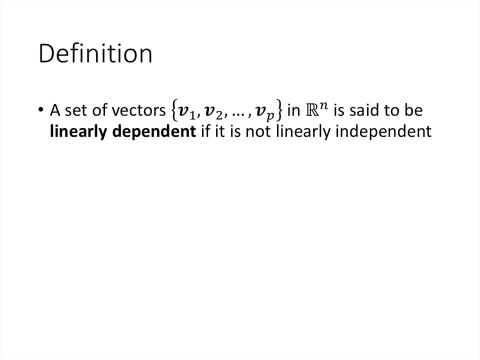 In this case we found lots of solutions. so that means that the vectors are not linearly independent. So this gives us another piece of terminology. We can flip around the definition of linear independence and talk about what it means for a set of vectors to be linearly dependent. So, linearly dependent. 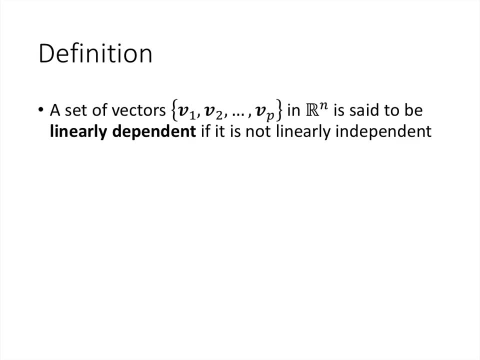 just means not independent. It's the opposite of the word independent. We can be more specific though, Putting in the definition of linear independence. if we say that the linearly dependent means that the vectors are not linearly independent, then that just means that that vector equation has a non-trivial 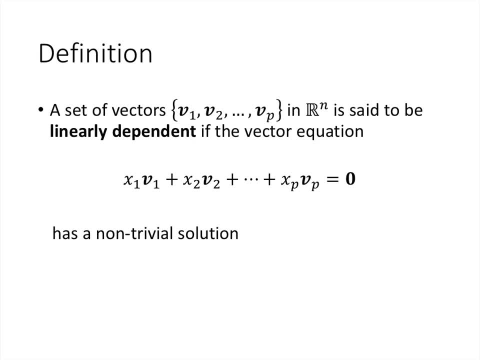 solution. Remember, linear independence means that the only solution is the trivial solution. So linearly dependent would mean that there is at least one other solution other than the trivial solution. Being a little bit more specific, what linearly dependent means is that there 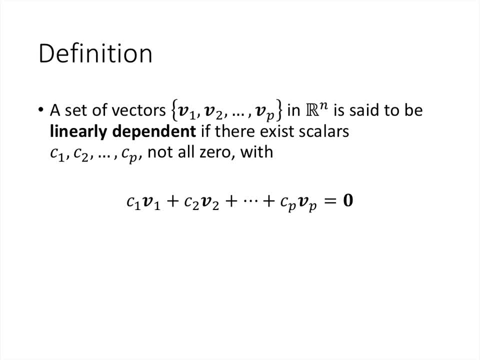 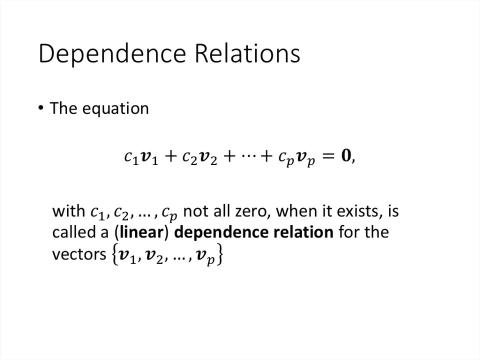 exist- numbers that are not all zero- Some of them might be zero but they're not all zero- that we could plug in for the x's to make that linear combination end up being the zero vector. And this equation here has a special name: We call that. 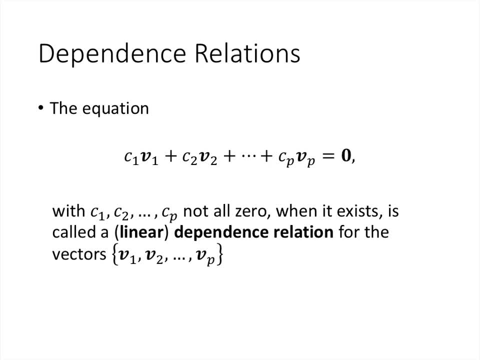 equation, a dependence relation or a linear dependence relation for those vectors. If there's some way to plug in numbers for the x's that are not all zero, we can use that equation to make the left hand side equal the right hand side. That way of doing that is called a dependence relation And in general for a. 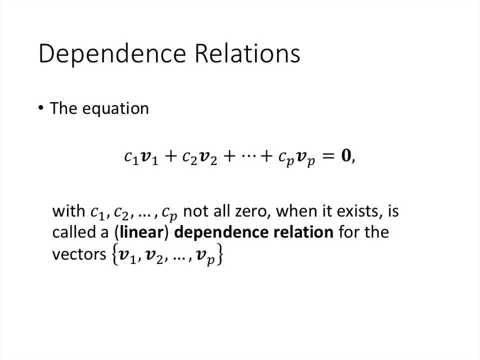 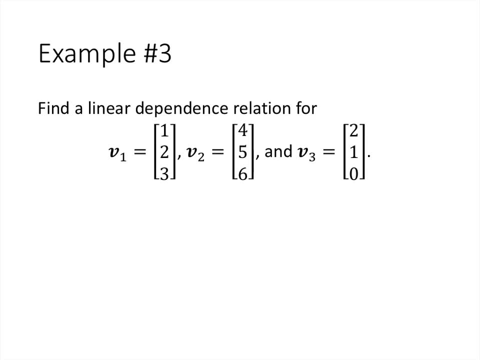 set of vectors that are linearly dependent. there are lots of ways to do that. Let's do an example. So here we have three vectors. Now I'm telling you that these vectors are linearly dependent, although we'll see that for ourselves as 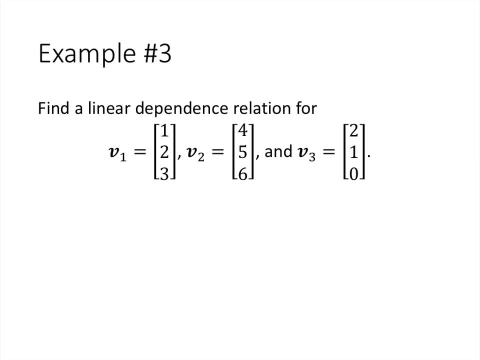 we go through this example. But given these three vectors, what we want to find is a linear dependence relation And all that means is a non-trivial solution, in other words, not all zeros to the vector equation. x1, v1 plus x2, v2 plus x3, v3 equals the zero vector. So let's plug in our vectors, Our 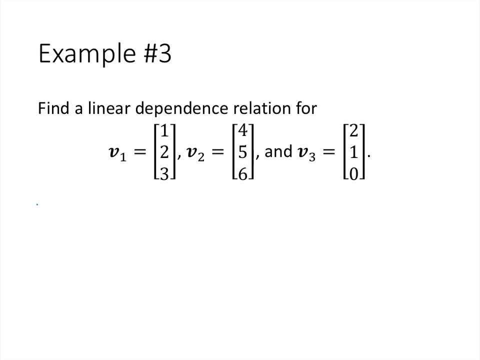 dependence relation, and all that means is a non-trivial solution, in other words, not all zeros to the vector equation. x1, v1 plus x2, v2 plus x3, v3 equals the zero vector. So let's plug in our vectors. Our first vector is our second. 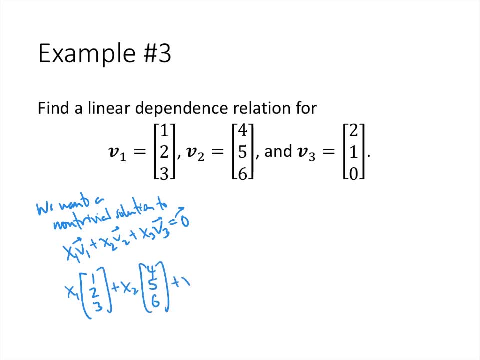 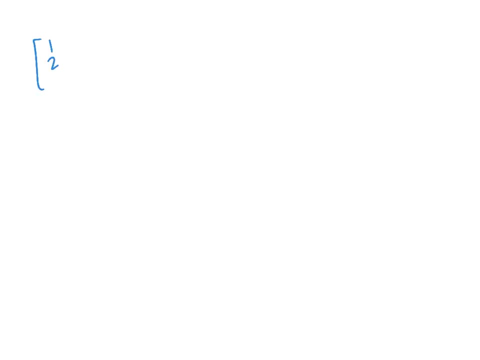 vector is, our third vector is: and we're setting that equal to the zero vector. So once again we're gonna set up our augmented matrix and row reduce. So our augmented matrix would be: We've got a 1 in the first row, first column, so that's good. Multiply first row by negative 2 and add. 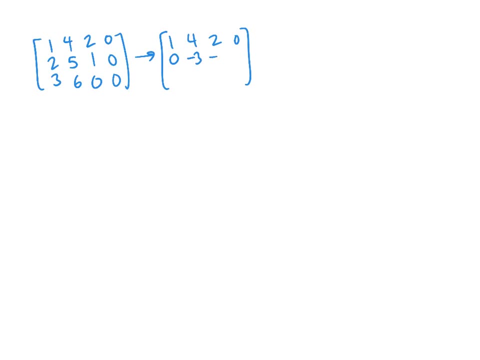 that gives us a zero. Negative 3, negative 3, zero. Multiply the first row by negative 3 and add. that gives us a zero. Negative 6, negative 6, and zero. Now we're gonna divide row 2 by negative 3,. 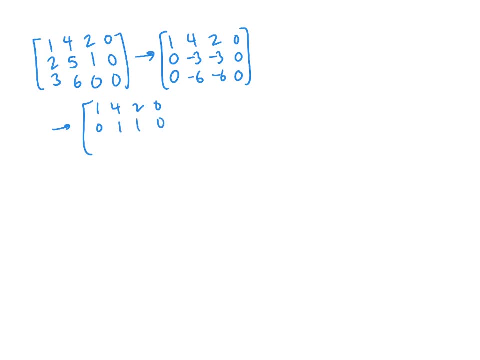 and now we're gonna fix that second column. Multiply row 2 by negative 4 and add it to the first row, that gives us a zero negative 2, and zero. Multiply row 2 by 6 and add it to the third row, that's gonna give us a zero, zero and zero. 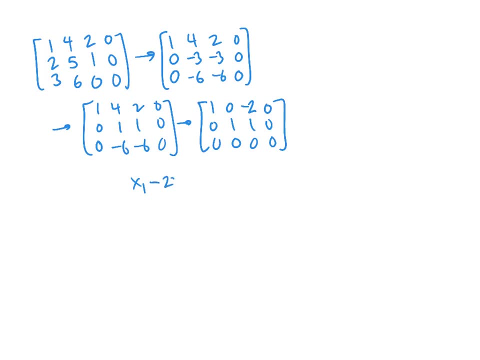 So this means that our solution is that x1 minus 2x3 equals zero, x2 plus x3 equals zero and x3 is a free variable. Solving for our variables, we get x1 equals 2x3,, x2 equals negative x3, and x3 is a free variable. 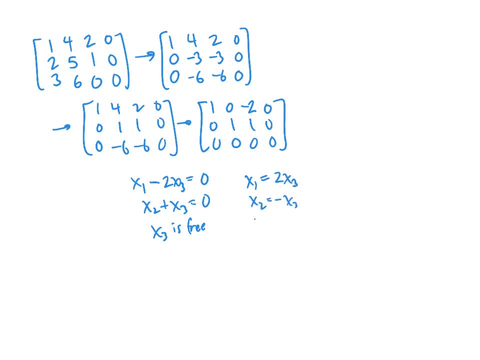 Solving for our variables, we get x1 equals 2x3,, x2 equals negative x3, and x2 equals negative x3. And x3 is free. So any value of x3 that we want to choose here will work to give us a dependence relation. 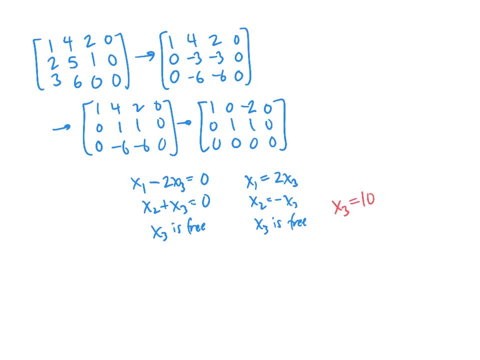 Let's use x3 equals 10.. I'm just picking a number at random, so I just decided that I'm gonna choose x3 equals 10.. If you like a different value, go ahead and use it. You will also get a good solution to this problem. 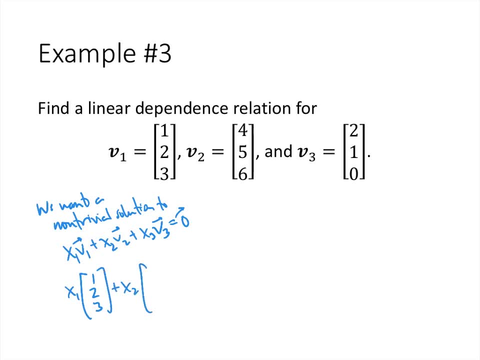 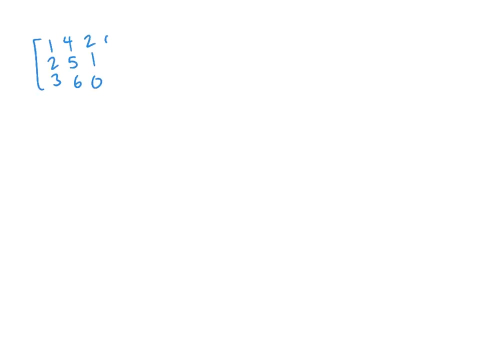 first vector is, our second vector is, our third vector is and our fourth vector is, and we're setting that equal to the zero vector. So once again, we're gonna set up our augmented matrix in row reduce. So our augmented matrix would be 1, 2, 3, 4, 5, 6, 2, 1, 0, 0, 0, 0.. 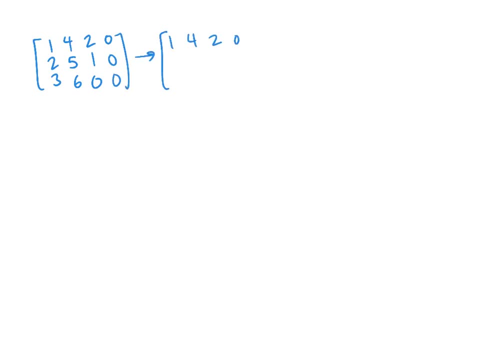 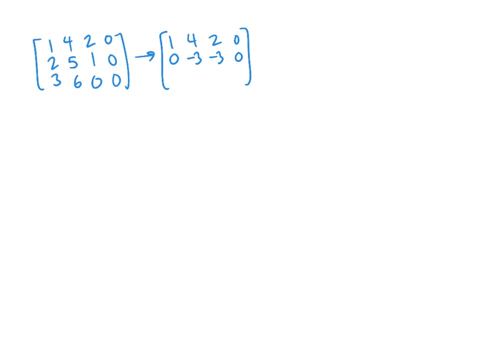 0.. Multiply the first row by negative 3 and add. that gives us a 0, negative 6, negative 6, and 0.. Now we're going to divide row 2 by negative 3, and now we're going to. 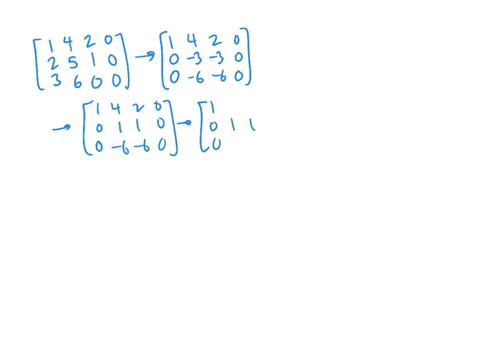 fix that second column. Multiply row 2 by negative 4 and add it to the first row: it gives us 0, negative 2, and 0.. Multiply row 2 by 6 and add it to the third row, that's going to give us 0,, 0, and 0.. So this means that our solution is that x1 minus 2x3. 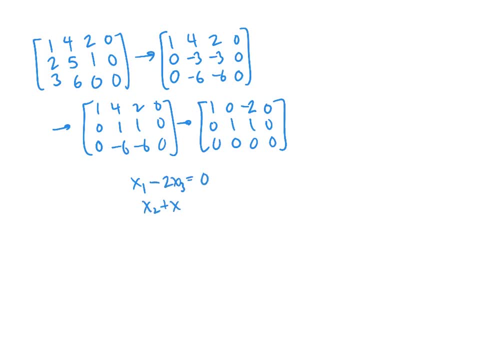 equals 0,. x2 plus x3 equals 0, and x3 is a free variable. Solving for our variables, we get x1 equals 2x3,, x2 equals negative x3, and x3 equals negative x3. 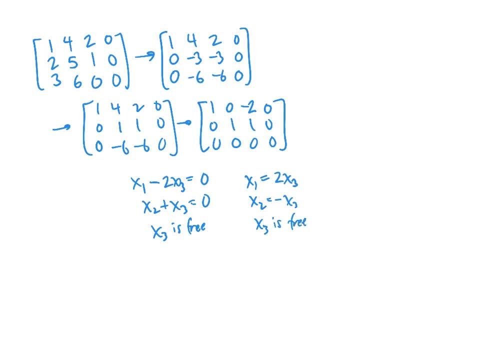 So any value of x3 that we want to choose here will work to give us a dependence relation. Let's use x3 equals 10.. I'm just picking a number at random, so I just decided that I'm going to choose x3 equals 10.. If you like a different value, go ahead and use it. You will. 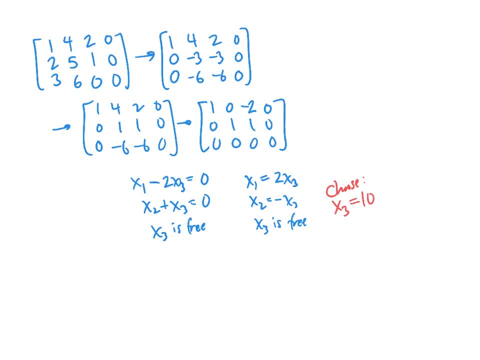 also get a good solution to this problem. So remember that a dependence relation is a way to put in numbers coefficients to these vectors and a number to these vectors, so that the left-hand side equals the right-hand side. So I'm going to put a number in this spot. 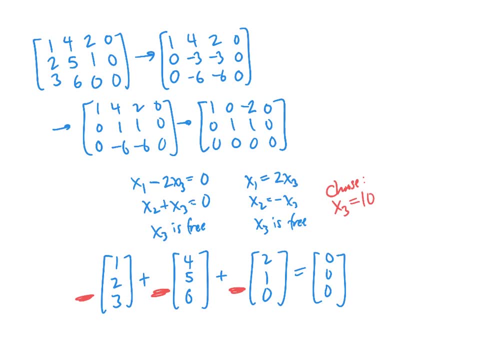 I'm going to put a coefficient here. and I'm going to put a coefficient here. So if I chose, x3 equals 10, well, x1 equals 2 times x3, so 2 times 10, which is 20.. 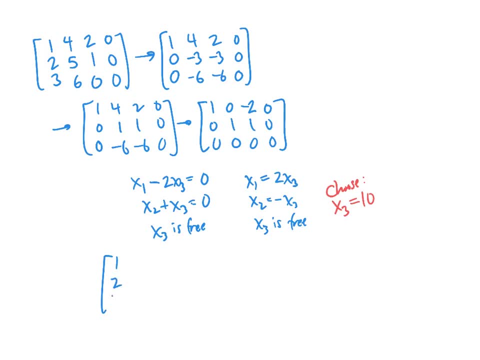 So remember that a dependence relation is a way to put in numbers coefficients to these vectors, so that the left-hand side equals the right-hand side. So I'm going to put a number in this spot, I'm going to put a coefficient here and I'm going to put a coefficient here. 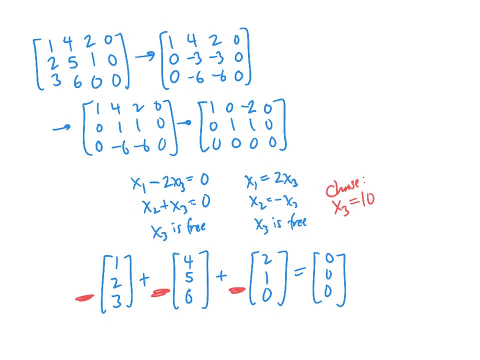 So if I chose x3 equals 10, well, x1 equals 2 times x3,, so 2 times 10, which is 20.. Since I chose, x3 equals 10, x2 is negative x3,, so that's negative 10.. 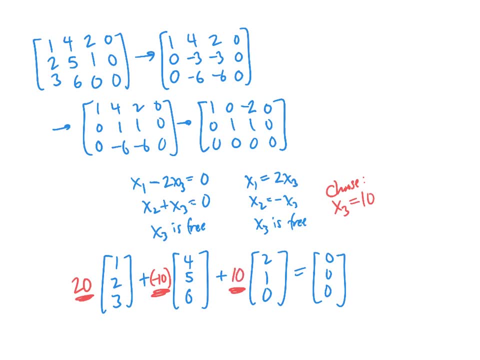 And x3 is 10, so that's what I put there. But again, if you don't have a dependent relation, you don't have a free variable. If you decided you wanted a different value, go ahead and choose it. If instead you said, you know what I didn't want: x3 equals 10, I want x3 to equal, let's say, 4.. 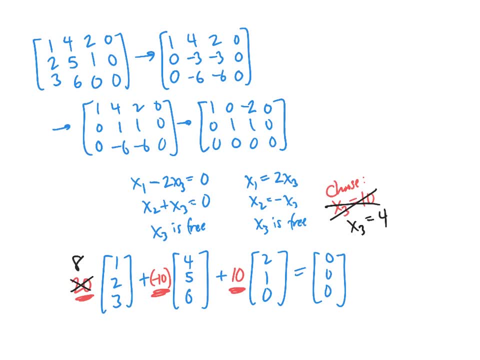 Well then, x1 equals 2x3,, so you would put an 8 here. x2 equals negative x3, so you would put a negative 4 here. And x3 equals 4, so you would put a 4 here. 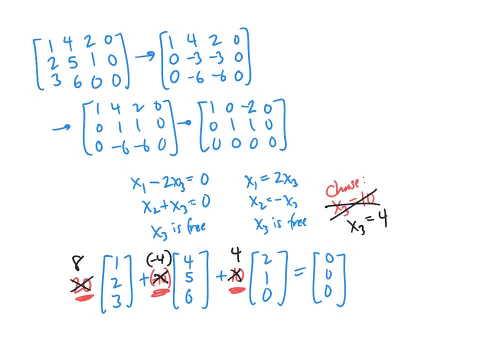 And your solution is just as good as my solution. In general, when there is a dependence relation, there are actually lots and lots of dependence relations, all of which could work. Subtitles by the Amaraorg community. Subtitles by the Amaraorg community. 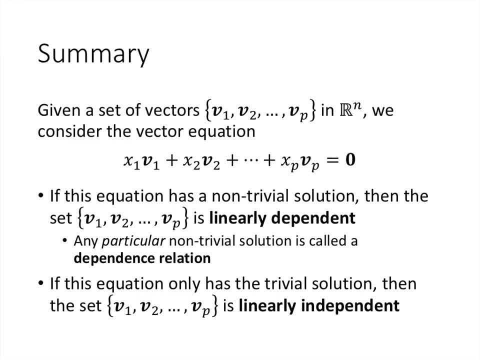 So just to wrap this up and again, this concept of linear dependence tends to be something that folks have a hard time wrapping their heads around. So feel free to watch this video multiple times. really pause it. think about the different examples. try to work through the examples on your own. 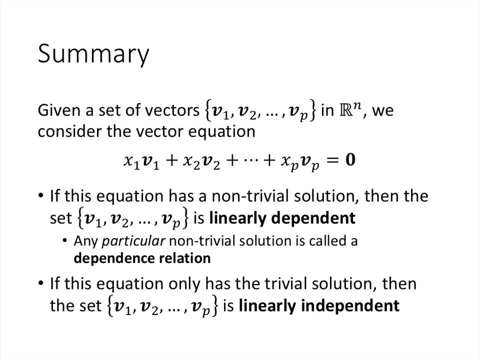 But here's the wrap-up: Given a set of vectors, we're looking at this vector equation: x1v1 plus x2v2 plus, plus, plus. all the way through xpvp equaling to the zero vector, All the way through xpvp equaling to the zero vector. 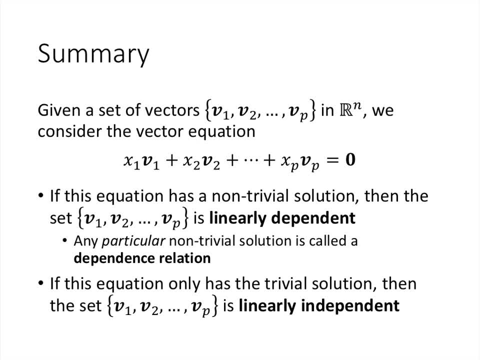 All the way through xpvp equaling to the zero vector. If that equation has a non-trivial solution, then we say that the set of vectors is linearly dependent And any particular non-trivial solution, any solution that we find other than all zeros, is called a dependence relation. 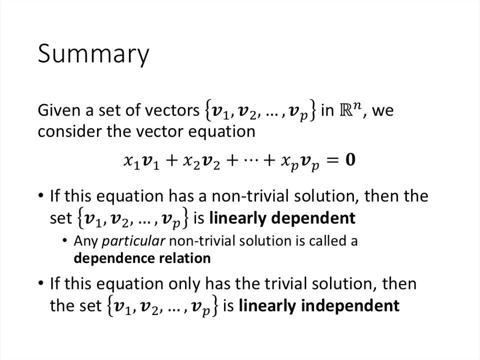 But if that vector equation only has the trivial solution, only has the solution where all of the x's equal zero, then we say that the set of vectors is linearly independent.